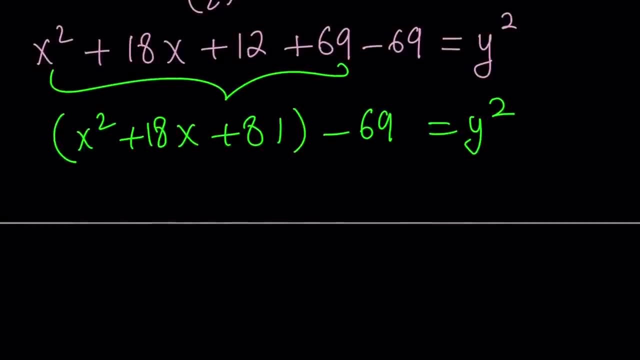 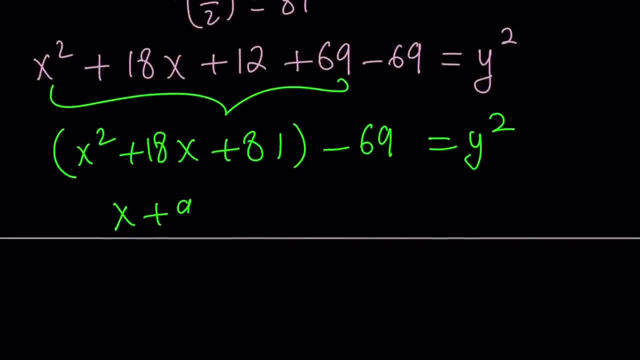 Now, inside the parentheses, we have a perfect square. That's perfect. So let's write it as x plus 9.. I don't know why this is disappearing. Okay, x plus 9 squared minus 69 equals y squared. Now, 69 is not a perfect square, but y squared is. 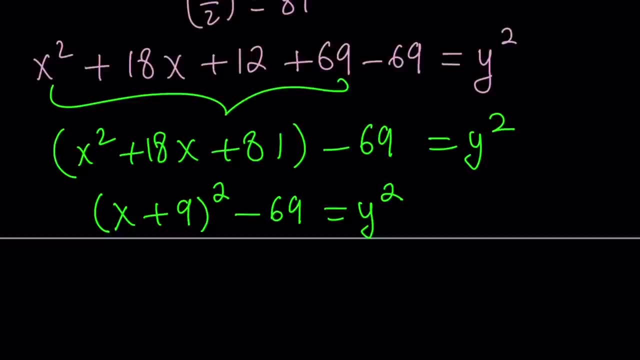 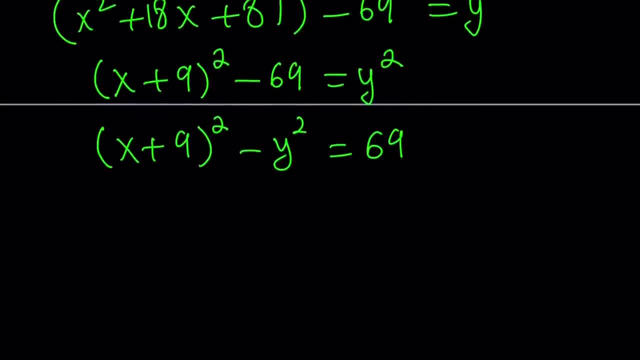 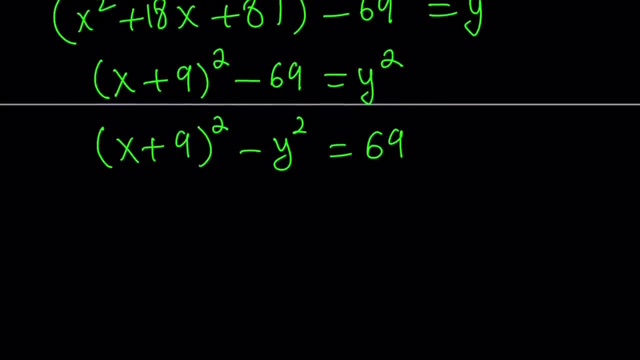 If you ask me what is one of the most important formulas or identities in math, I would say difference of two squares. The other one is probably the Pythagorean theorem. Anyways, let's go ahead and factor this. This can be written as: x plus 9 plus y times x plus 9 minus y equals 69.. 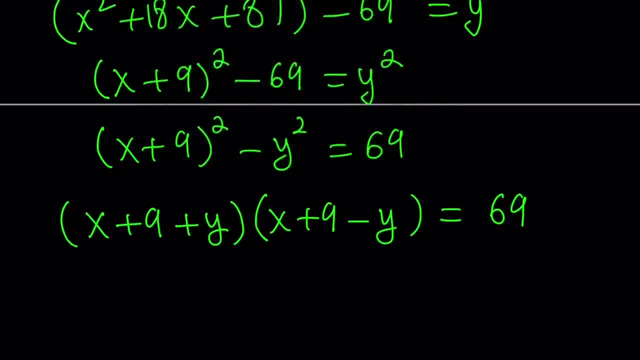 Awesome. Now we can go ahead and Look at factors of 69.. 69 is not prime, even though it's somewhat prime looking. Notice that 6 and 9 are both divisible by 3,, which means the sum of the digits of 69,. 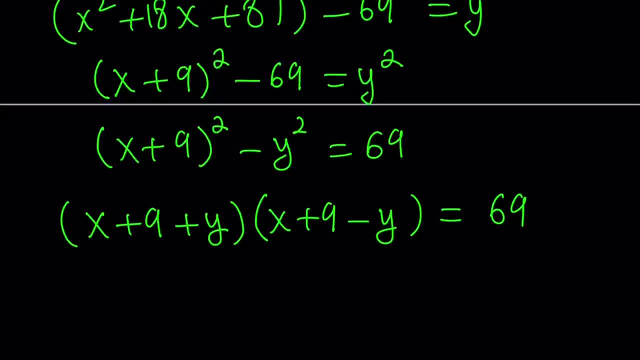 which is 15, by the way, is a multiple of 3, which means 69 is a multiple of 3.. And it's in fact 3 times 23,, which is kind of interesting because 69 can be written as the product of two primes. 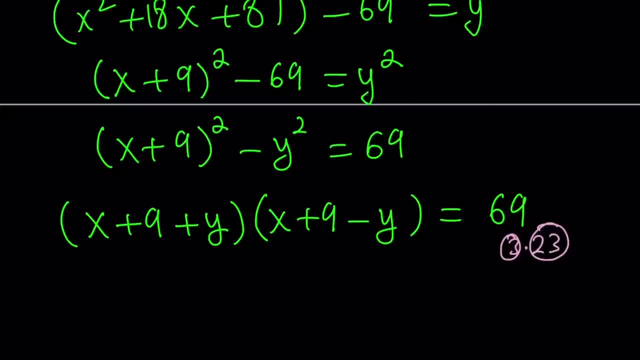 That tells you that it has four positive divisors. Great, Okay, great. Let's go ahead and take a look at each case, And now we're going to be finding the x and y values from here, But early on we can safely say that there's going to be eight solutions, because if you 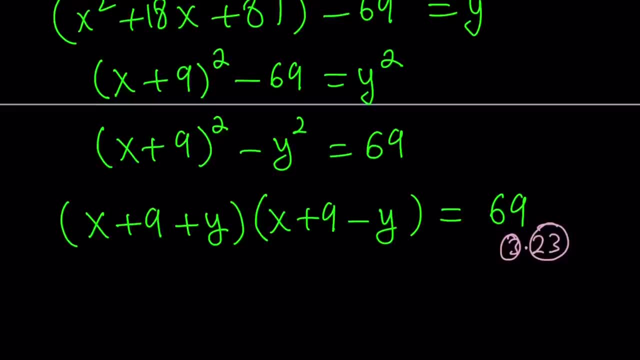 consider the negatives. they're going to give you eight solutions, But let's go ahead and walk through each solution. And now we're going to look at the results from alpha. Let's see if from alpha can find all the solutions And then we'll look at. 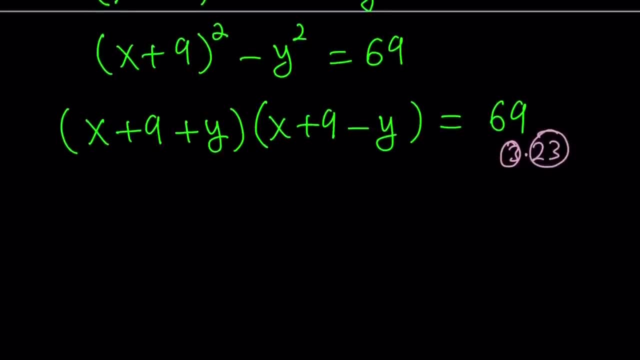 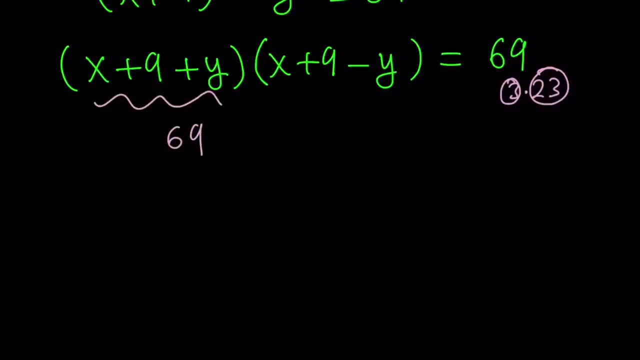 Let's look at a graph real quick. Okay, now, these are some- not some, but all the cases. pretty much, We can basically set this equal to 69 and set this equal to 1.. Now, what does that entail? 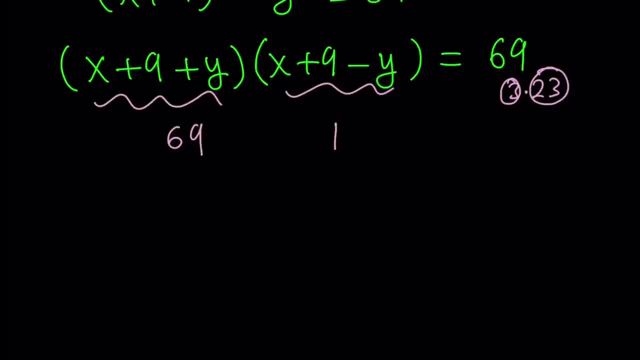 Well, if you set this equal to 69, that basically means that you're basically writing it as x plus y is 60 and x minus y is negative 8. So you get a system of equations right, And then you can easily solve it just by adding these two equations side by side. 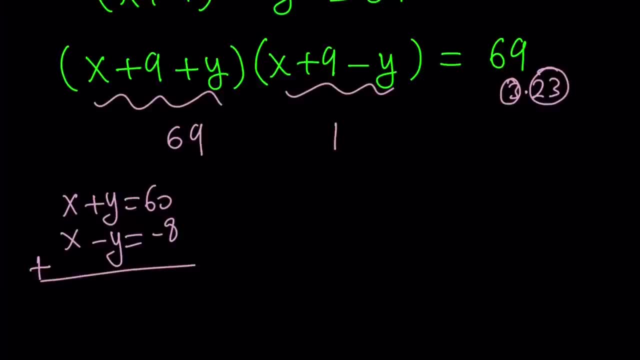 And then you're going to get 2x, which you can divide by 2,, and you're going to get x values. So from here we get 2x equals 52 and x equals 26. But if you plug in 26,, that gives you y equals 34.. 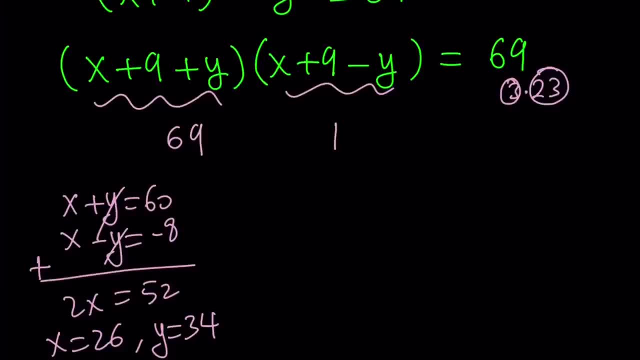 So we basically get an ordered pair from here which we can write as 26 comma 34.. So that's That's an easy system to solve because it's linear and you can just go ahead and apply it to all the different cases. 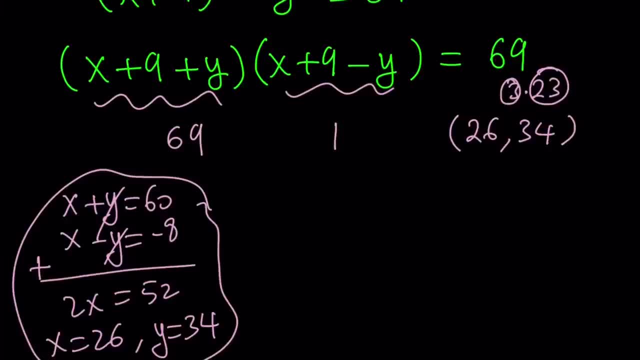 But to keep a long story short, I'm not going to do all the system solving here because that's going to take a long time. and you can do it, It's going to be good practice. I'll just give you the ordered pairs based upon what we get from factors. 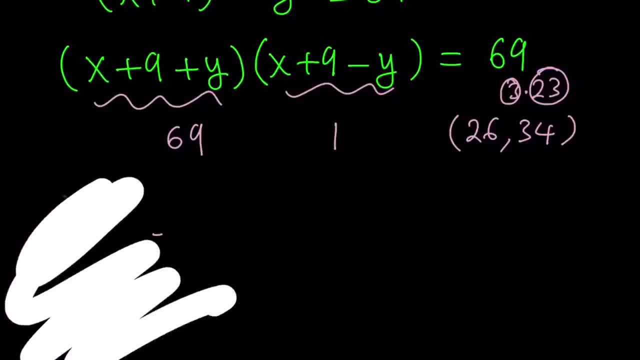 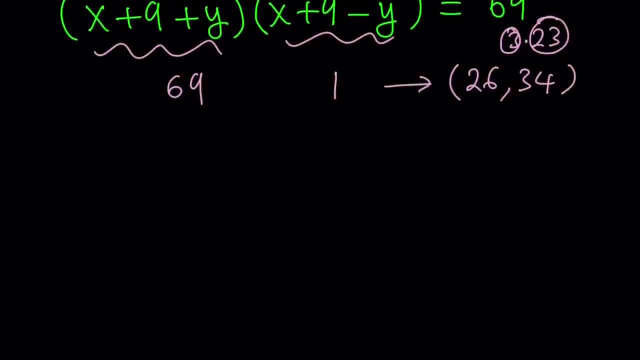 Okay, anyways, let's go ahead and clear this up. And now we're going to write each possibility and look at the corresponding ordered pair. So 69 times 1.. And then we can write 23 times 3.. And I want to go systematically, while decreasing the first factor and increasing the second. 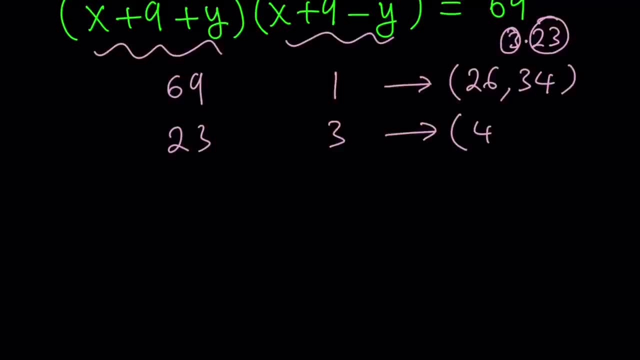 factor. So this is going to give us 4 comma 10.. And then I have 3 and 23.. Obviously, this can be switched, And something interesting happens: when you switch this, You're going to get the ordered pair 10 comma 4.. 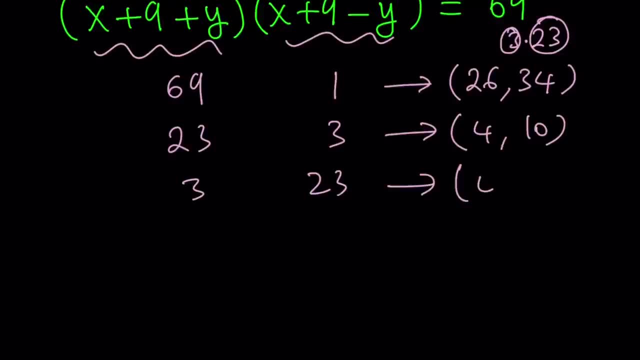 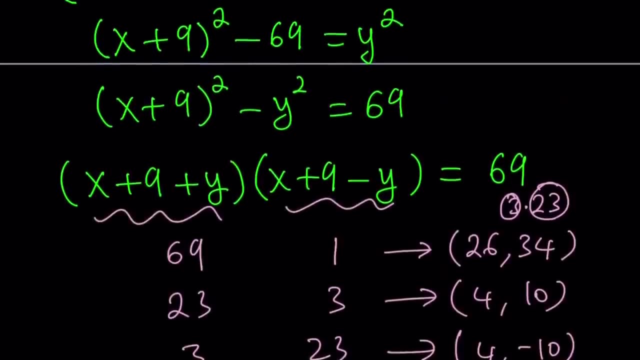 Actually not 10 comma 4.. It is going to be the 4 comma negative 10.. Okay, so here's what happens. Let me tell you what is going on. I know Most of you thought about this. Since y is squared, if y equals y sub 0 is a solution. negative y sub 0 is also a solution. 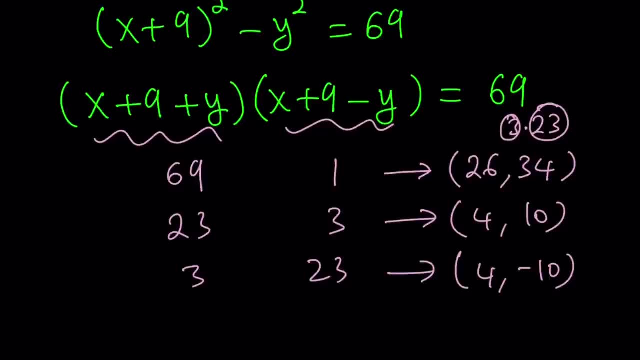 Because when it's squared it's going to give you the same result. So y is going to come with two signs. plus minus Make sense, Okay, great, But x values are going to be pretty much fixed. So the next one, it's not too hard to guess. 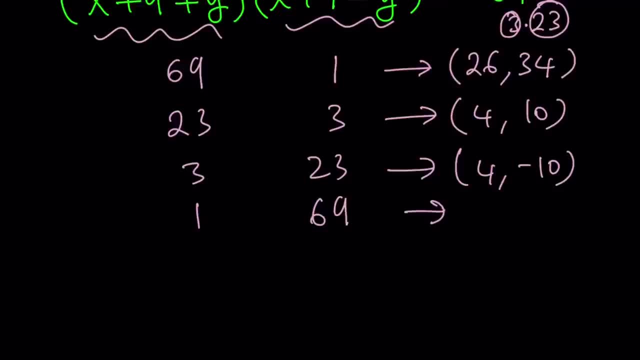 If you go with 1 and 69, this should give you pretty much the same thing as the first one, Except y is going to be negated. Make sense, Okay? So those are the first four, And then now we can look at the negative factors, like negative 69 and negative 1.. 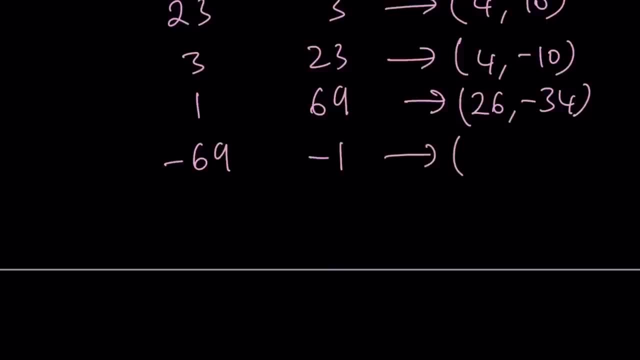 And then this is going to give us negative 44 and negative 34.. Both of them are going to be negative in this case. And then we have the negative 23 and negative 3.. This is going to give us negative 22 and negative 10.. 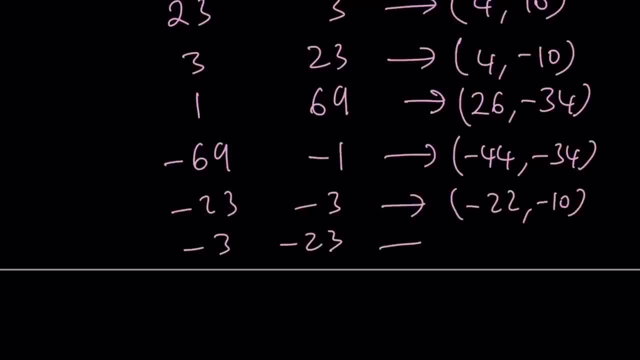 And then we have negative 3 and negative 23.. Obviously not too hard to guess right. Same thing, pretty much: Y value will be negated. And finally we have the negative 1 and negative 69, which is going to be negation of y on. 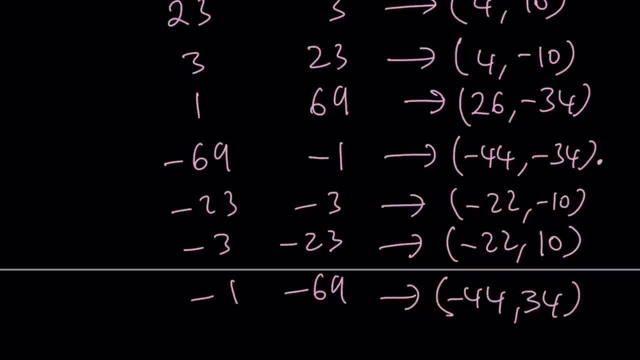 this ordered pair: negative 44,, positive 34.. So both x and y are negative for two cases, And then they're just going to switch around differently. Okay, so these are going to be all the solutions. Hopefully you can see them all together like this, right. 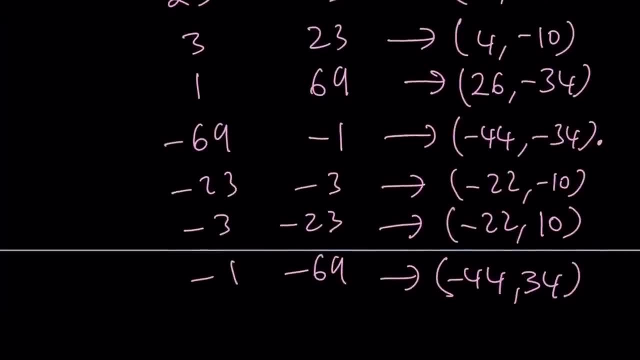 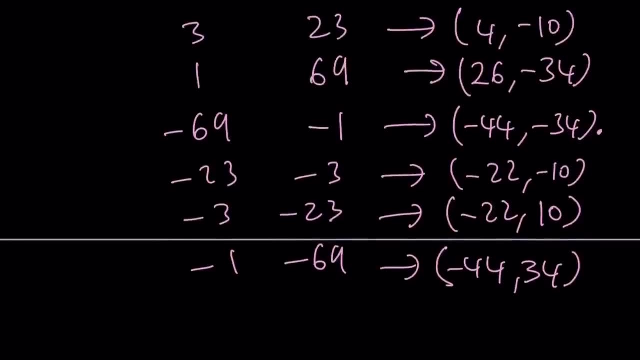 Okay, And then We're going to just go ahead and look at what Wolfram Alpha gave us, And then we'll compare. if you can get eight results from there too, All right, And then we'll look at the graph and we'll finish up real quick. 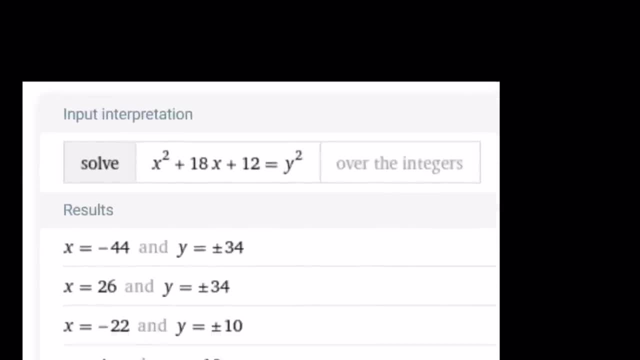 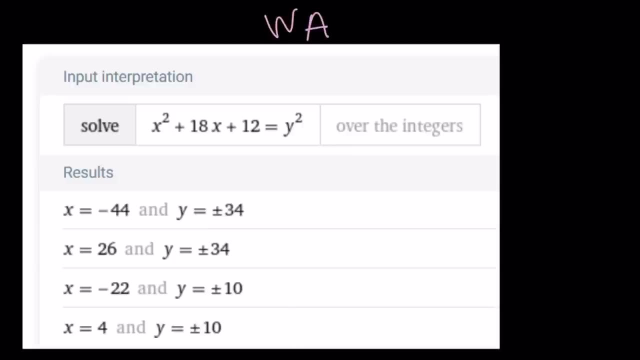 All righty. So here's the result from Wolfram Alpha. If you enter this, you know it's great, It's a really great tool And you can basically go to wolframalphacom and enter the same equation And, as you can see here, we get eight solutions. 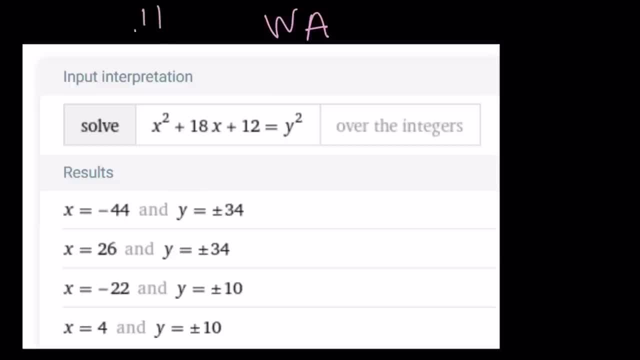 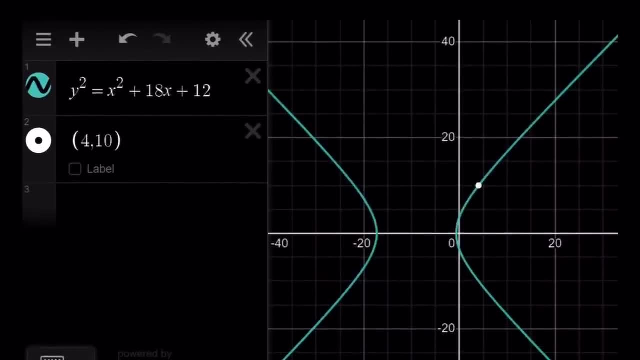 So you can see that we have a solution with the plus minuses. Awesome, Good job, Wolfram Alpha. Let's go ahead and take a look at the graph. This is the graph of a hyperbola. Why is it a hyperbola?